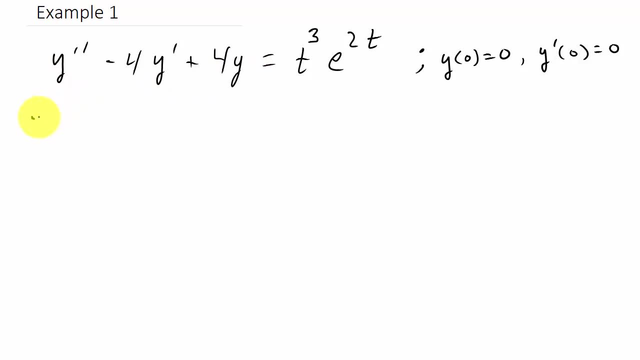 to take the Laplace transform of each term, So that's going to be the Laplace transform of y double prime minus the Laplace transform of this, and I'm going to bring the four out. So that's four Laplace transform of y prime plus, and then I'm going to bring this four. 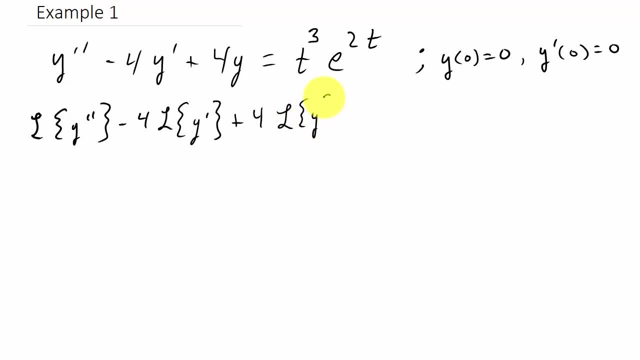 out four. Laplace transform of y equals the Laplace transform of t cubed e to the 2t. Alright, so the way we write this equation is: we're going to take the Laplace transform. what we rewrite the Laplace transform of y double prime is s squared y of s minus s. 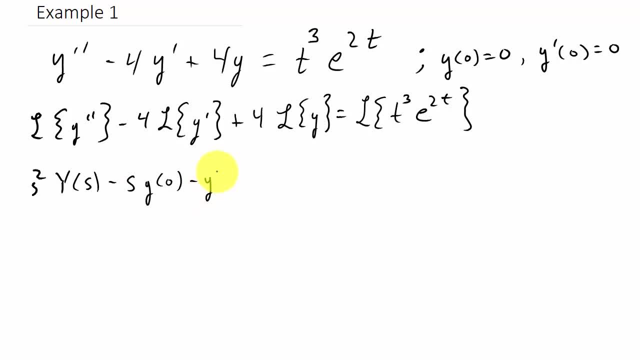 times y of zero minus y prime of zero, And then we rewrite this one, so that's minus four, and then that's going to be s, So that's y of s minus y of zero, And keep in mind that it's minus four times this. so 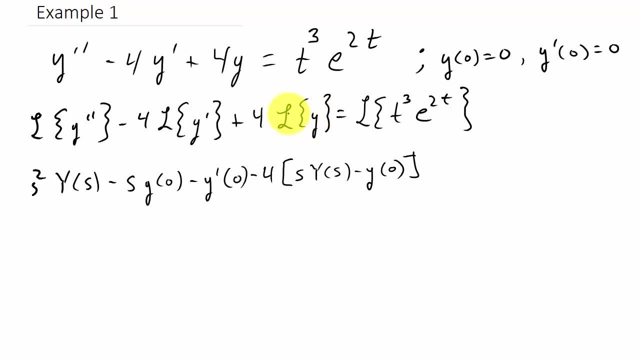 that's why we have this in parenthesis. And then the Laplace transform of y. that's just going to be plus four, and then Laplace transform of y is y, s And that equals alright. so we're going to take the Laplace transform of t, cubed e to the 2t, And then we rewrite. 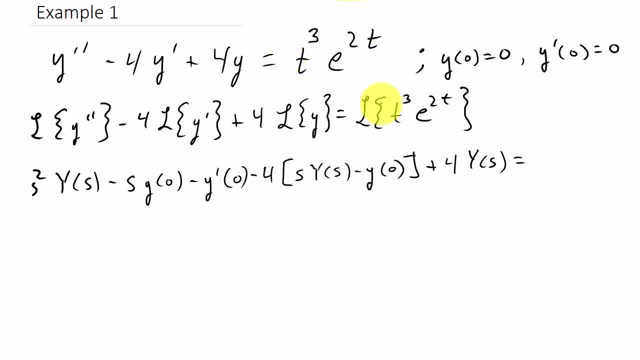 that one, Alright. so now let's take a look at this. We have a formula that says the Laplace transform of t to the n at is equal to n factorial over s minus a raised to the n plus 1.. So you can see here that n is equal to the number of times s plus 1. So that's equal to n factorial. 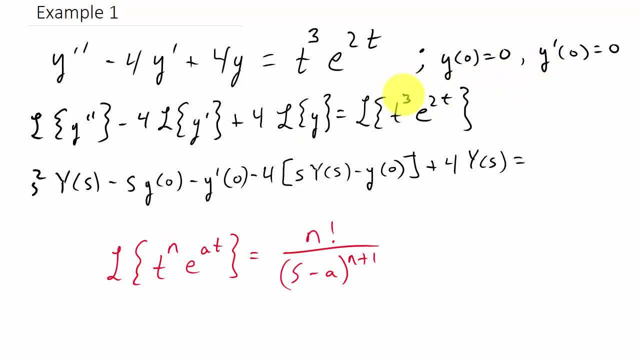 over s minus a, raised to the n plus 1.. So that's equal to n factorial over s minus a persons. Ok, See, that's my exponent here. n is 3, so that's 3 factorial over and then a. okay, you see the a, that's 2, so that's s minus 2, and that's raised to the n plus 1.. 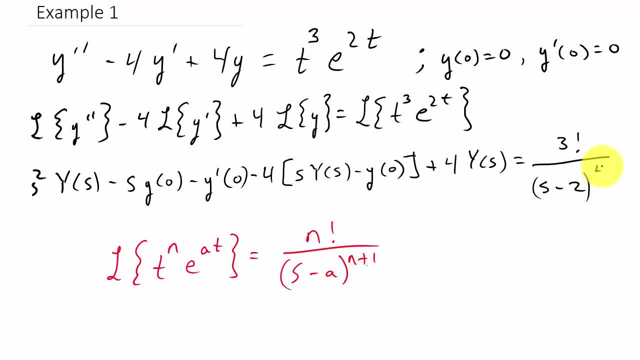 Well, n is 3,, so that's going to be 3 plus 1,, which is 4.. All right, so let's get rid of this. All right, so now what we need to do is we need to isolate the y of s, okay. 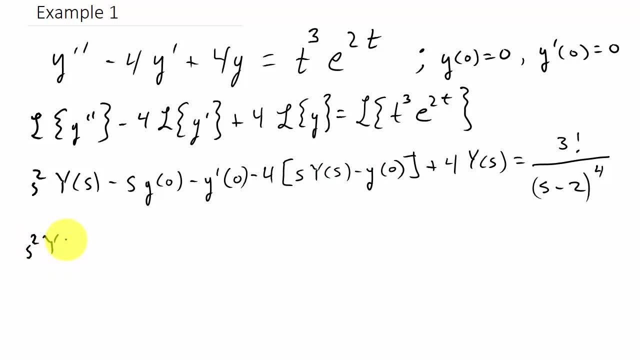 So that's going to be s squared times y of s minus s times y of 0.. Well, y of 0 is just 0.. y of 0 minus, and then y prime of 0 is 0, minus 4 times this s y of s. so that's 4s y of s, and then y of 0 is 0, so negative 4 times 0 is just 0, and then plus 4y of s. 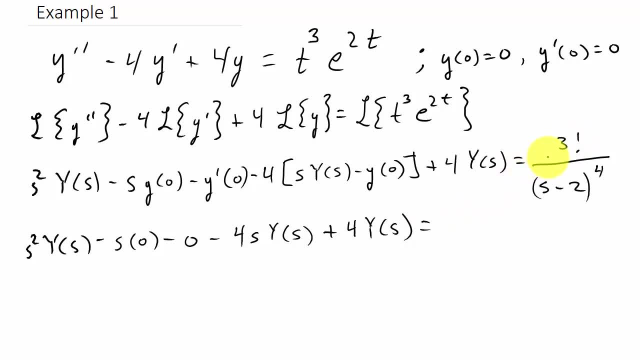 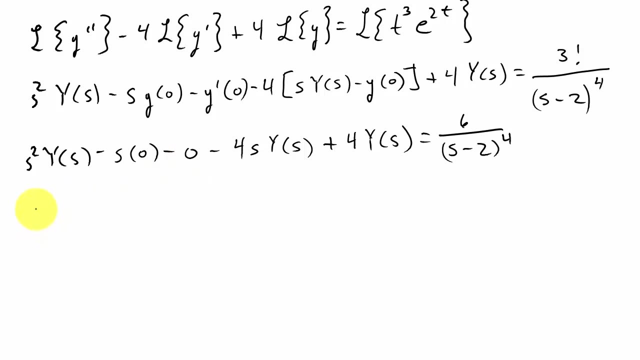 And that equals well 3 factorial, and that's 3 times 2.. times 1,, which is 6, over s minus 2 to the 4th. All right, so this term goes out, and this term goes out, and I'm left with s squared: y of s minus 4s, y of s plus 4y of s equals 6 over. 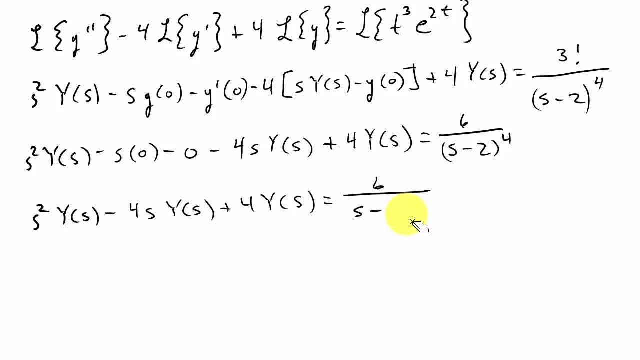 s minus s, minus 2 to the 4th. All right, so now what I'll do here is I'll factor out the y of s, So that's y of s times s squared minus 4s plus 4 equals 6 over s. 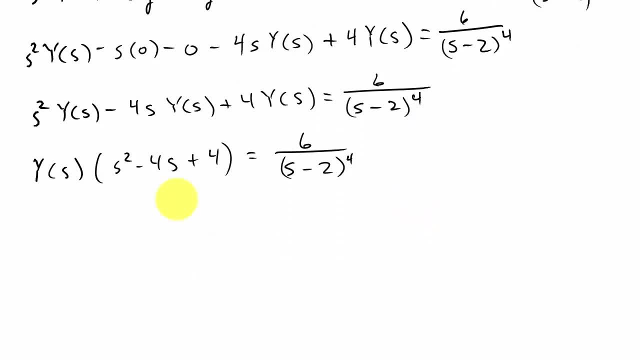 minus 2 to the 4th and then look at this: This will factor, and this is a. this will factor into y of s times: s minus 2 squared equals 6 over s minus 2 to the 4th. 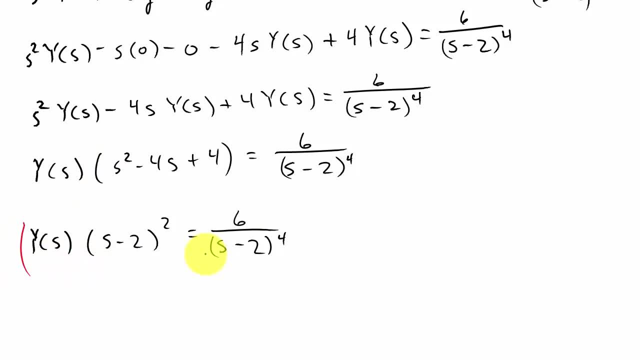 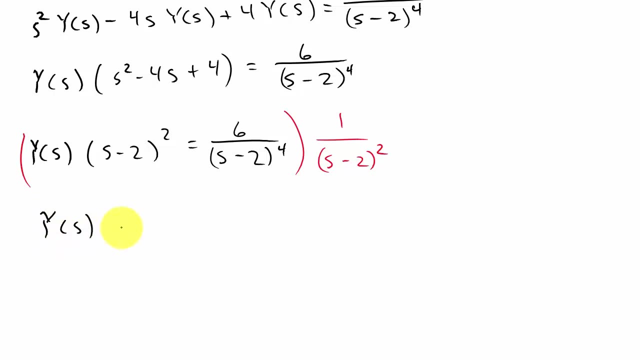 And now what I'm going to do is I'm going to multiply everything by 1 over s minus 2. squared, and that'll get rid of this term here. Okay, so that's going to give me y of s equals 6 over. 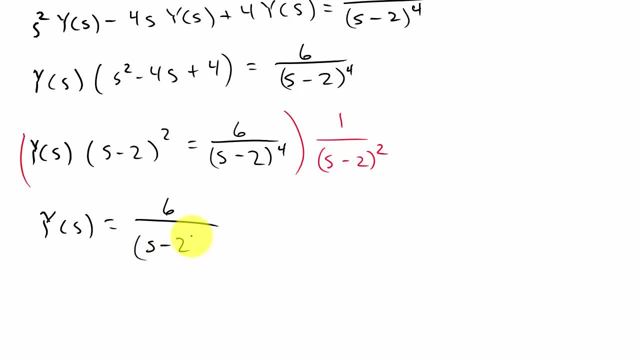 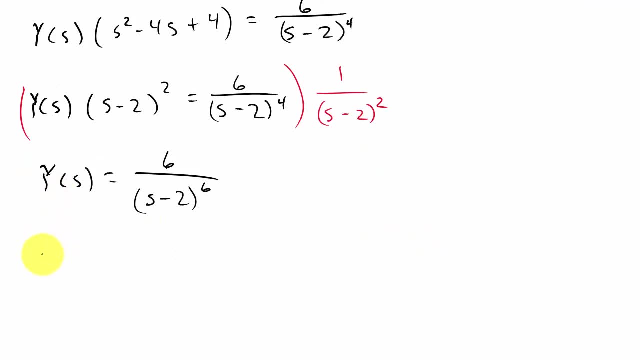 and then, when I multiply this, this is s minus 2 to the 6th. All right, so now I have y. of t is equal to the Laplace transform of this, this side 6, over s minus 2 to the 6th. 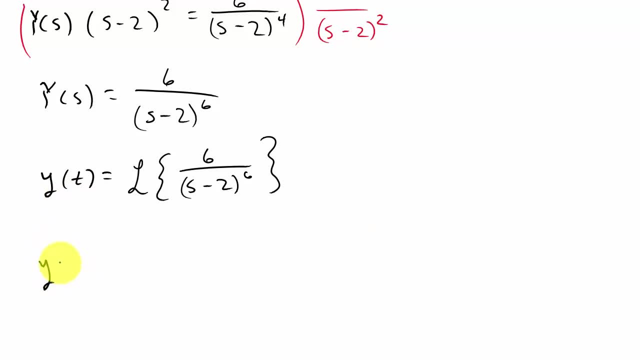 All right. so what we'll do here is we'll have y of t is equal to- and I'm going to take the 6th and I'm going to bring it out. So that's 6 times the Laplace transform of 1 over s, minus 2 to the 6th. 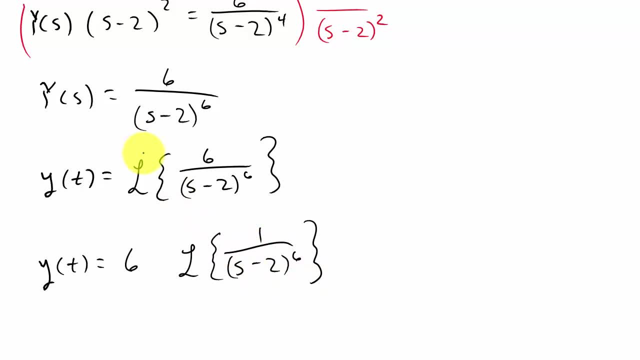 All right. so now I have to take. I'm sorry we're not taking the Laplace transform, we're taking the inverse Laplace transform. Sorry about that, All right. so look at this Well, remember from earlier the Laplace transform of t to the n. 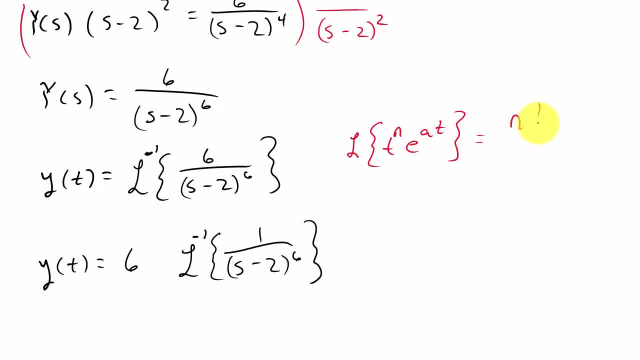 e to the at is equal to n factorial over s minus a to the n plus 1.. So this is what I have here. All right, so I have. n is well, first off, a is 2, okay, a is 2.. 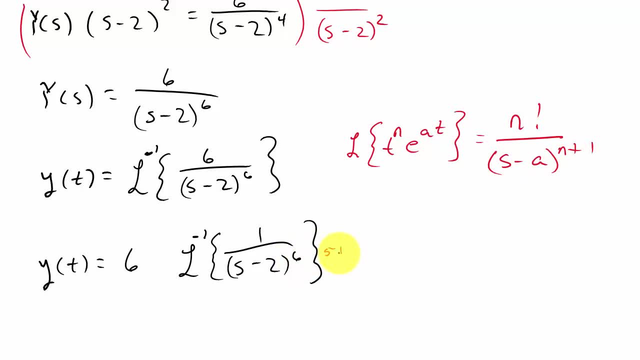 n. well, that would be 6, would be 5 plus 1, so n is 5.. Well, I need an n factorial up here, so that means I need a 5. 5 factorial, so that. so I multiply by the 5 factorial. 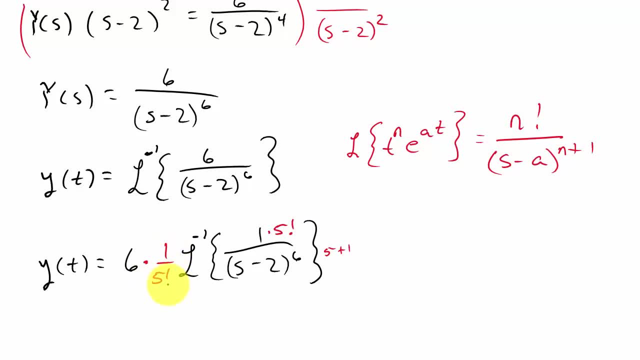 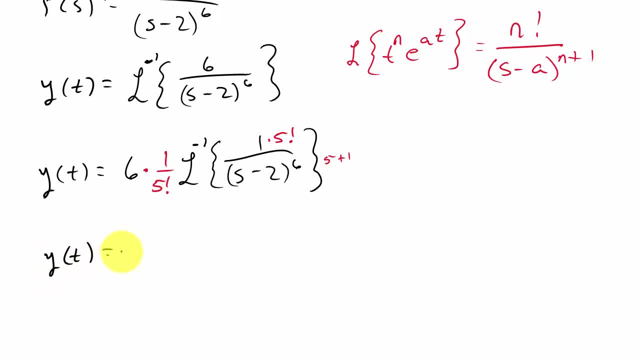 so that means I have to come out here and multiply by 1 over 5 factorial, And so now I have: y of t is equal to, and then 6 over 5 factorial. well, remember, 5 factorial is 5 times 4 times 3 times 2 times 1..